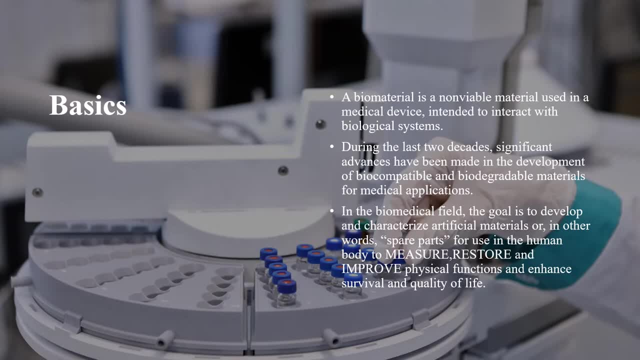 characterize certain artificial materials or in other words, the spare parts that can be used in the human body for measuring or restoring or improving the functions and also surviving the quality of life. So, basically, when a tissue or an organ is injured, so these can be utilized for restoring and improving the damaged and worn out functions. 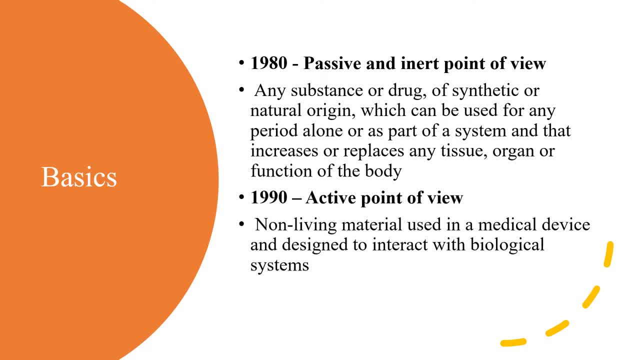 Giving an overview and basics of and history of it. So in 1980s the passive and inert point of view was seen. So basically, any substance or a drug which is of synthetic or of natural origin and that which can be used for any period, alone or as part of a 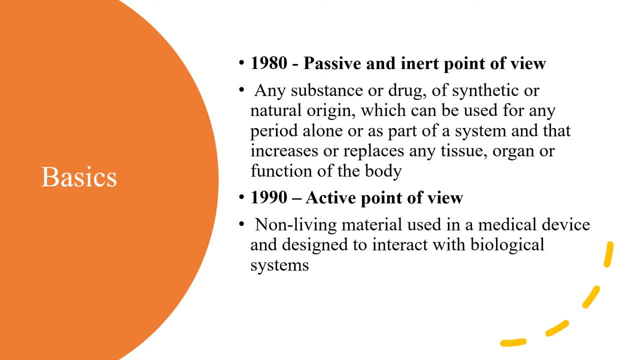 system and that increases or replaces the tissue, organ or function of the body, was termed as biomaterial. Further there were certain changes. after one decade, So around 1990s, there was a change in the form of a biomechanical material. So in 1990s there was a change in the form of a 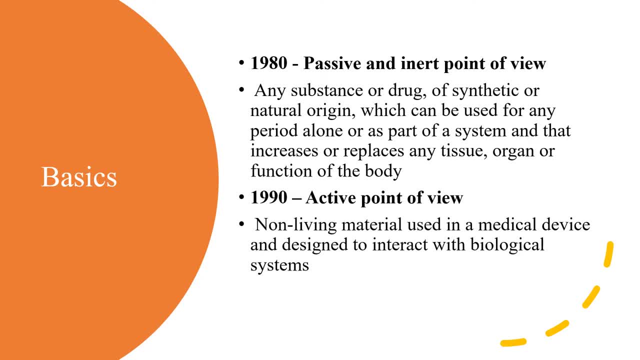 biomechanical material. So in 1990s there was a change in the form of a biomechanical material. So early 1990s the active point of view was considered and later the definition was a little bit changed and it was transformed into any non-living material that can be used in a 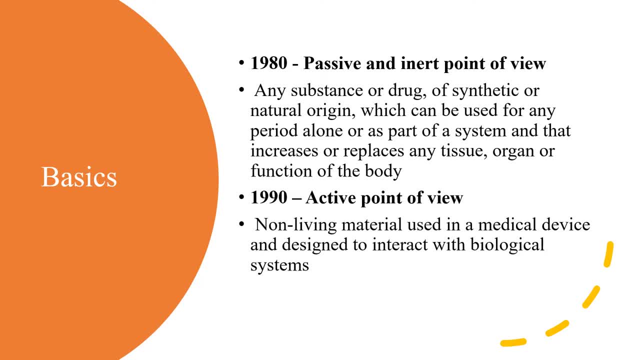 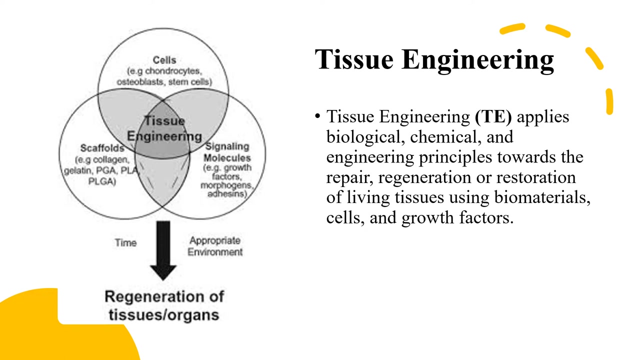 medical device and that is being designed to interact with the biological systems. So a biomaterial is termed as the material that can be utilized within the biological system and hence known as biomaterial, further brushing up the definition of tissue engineering. so our tissue engineering applies the biological, the chemical and engineering. 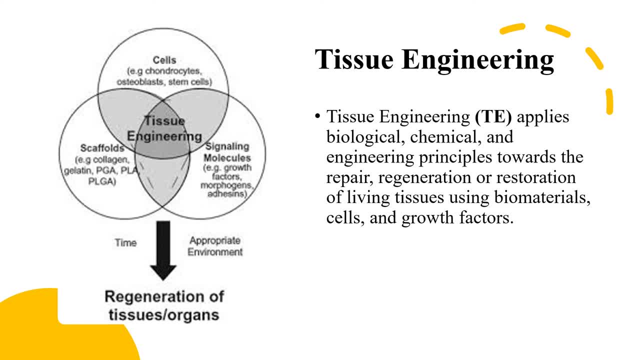 principles towards repairing, regenerating or restoring the living tissues by utilizing biomaterial, cells and growth factors. so there are major three components that are involved in tissue engineering, which are the cells of the scapules and the signaling molecules, or the other bioactive molecules that will help to regenerate the tissues and of the organs. now a one. 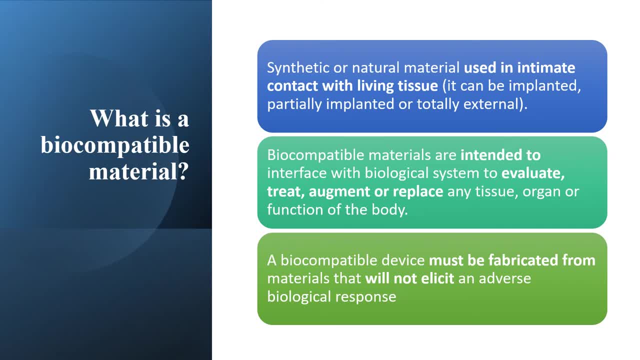 more term is there, which is the biocompatible material. so in one of my videos I have mentioned that there are certain characteristics and requirements for the material to be used in tissue engineering. so in this video I have showed you the real greenfield material that is also used in tissue. 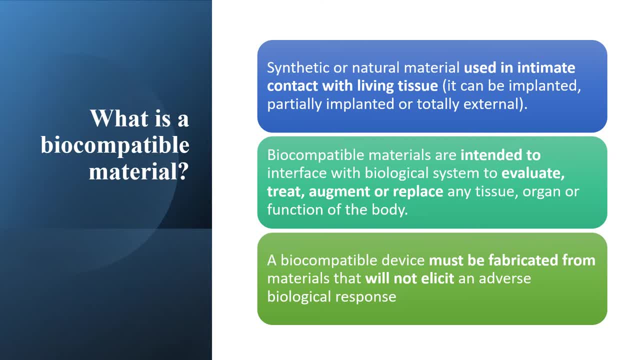 engineering, out of which one of the important criteria to be used as a biomaterial is the biocompatibility. so the material that is will be used should be compatible with the biological system, or else there will be reactions that will have a negative impact on the human body. so hence the 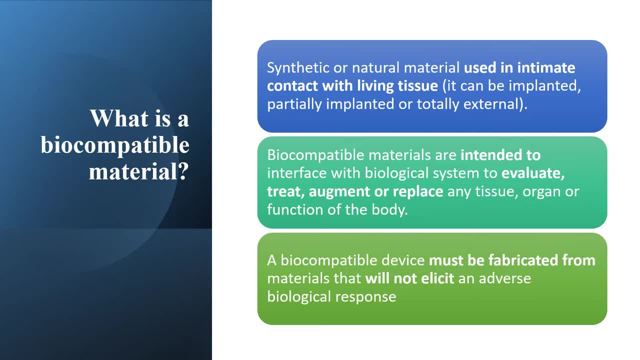 question arise is that what a biocompatible material is so any synthetic or natural material that is used in tissue engineering nodule composite material is used to put food starter in the tissue. sweaters. turbine equipment consumption. lleto Interview event is provided videos dedicated to physical results of the most common non-biμη Uses in tissue engineering from June 4-5 2020. 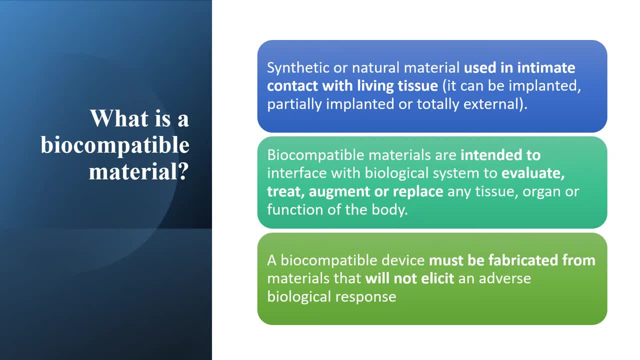 used in the intimate contact with the living tissue, That is, it can be implanted, partially implanted or totally implanted, or like which is ectopic or totally external, is known as biocompatible material. Further, biocompatible materials are intended to interfere the biological 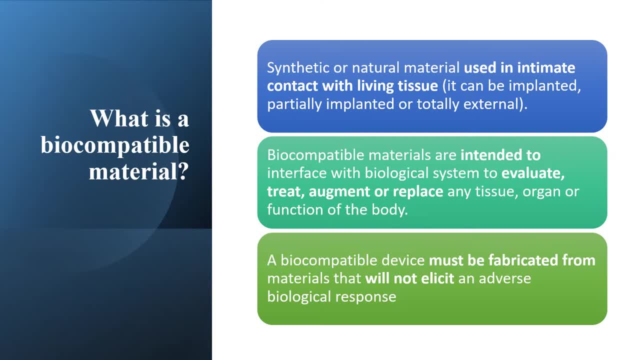 system in order to evaluate, treat, augment or replace any tissue, organ or function of the body, And then moving forward. so, basically, a biocompatible device must be fabricated from the materials that will not elicit or that will not give rise to any adverse immunological. 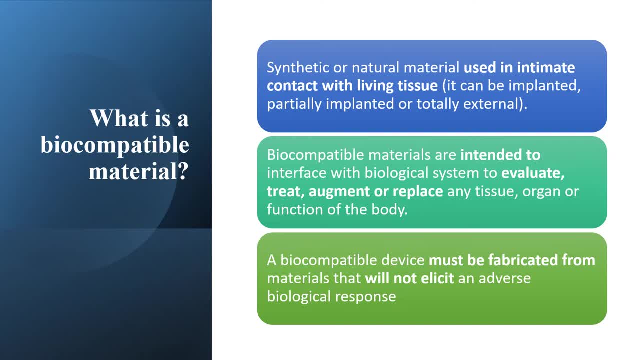 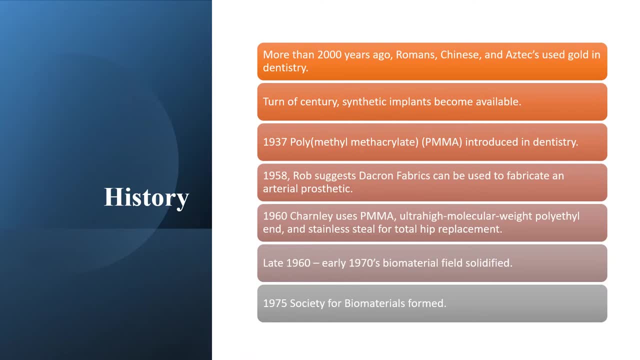 reactions and adverse biological response that can have a negative impact. Talking about the history of biomaterials, so more than 2000 years ago, raw material was produced in the form of a biocompatible material. So Romans, Chinese and Aztecs used gold in the dentistry. and the turn of century became when 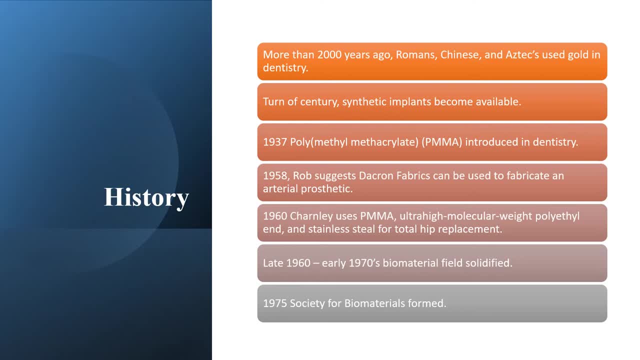 the synthetic implants became available. Around 1937, polymethylmethacrylate, which is also known as PMMA, was introduced into the dentistry field, And around 1958, Robb suggested that saccharine fabrics cannot be used to fabricate an arterial product. So the Chinese and Aztecs 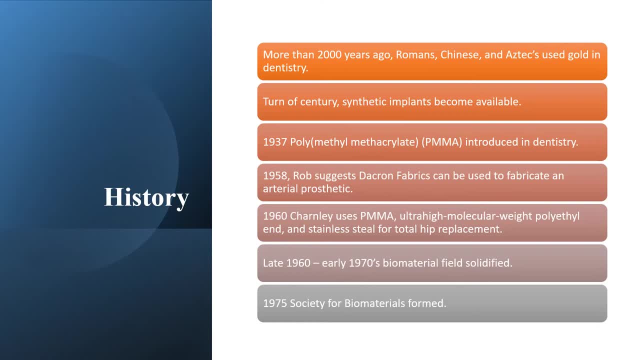 used polymethylmethacrylate. Therefore, in 1960, Charnley's used PMMA, which is ultra-high molecular weight, polyethyl end and stainless steel, for total hip replacement purposes. Later, in 1960s to early 1970s, biomaterial field further solidified and in 1975,. 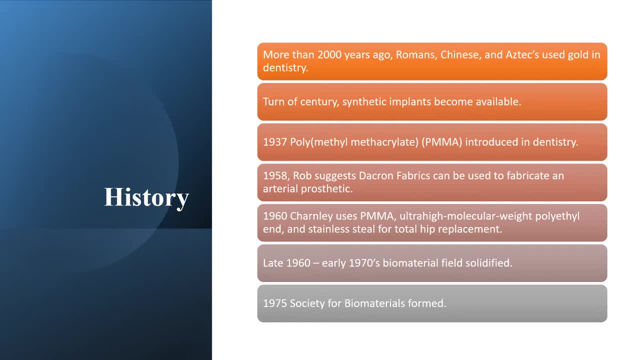 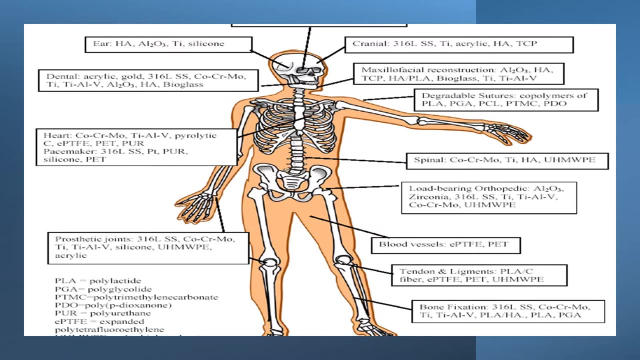 Society for Biomaterials was formed. This slide gives an overview of the history of biomaterials. This slide gives an overview about the different types of biomaterials that are used for different applications, For example, for the load-bearing orthopedic applications. various alloys of 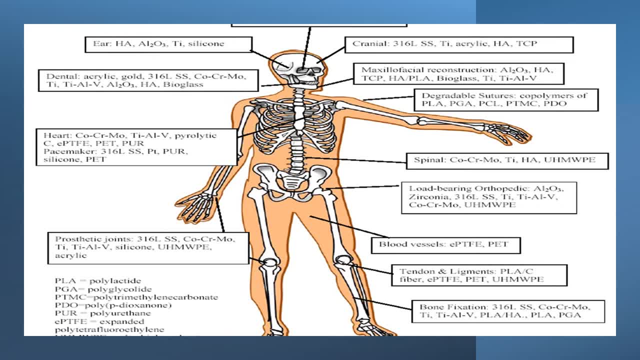 aluminium, zirconium and titanium-aluminium-valium are being used For certain cranial surgeries or for cranial recovery, certain stainless steel and then titanium-acrylic-hydroxyapatite-iocalcium-phosphate. these are being currently utilised. 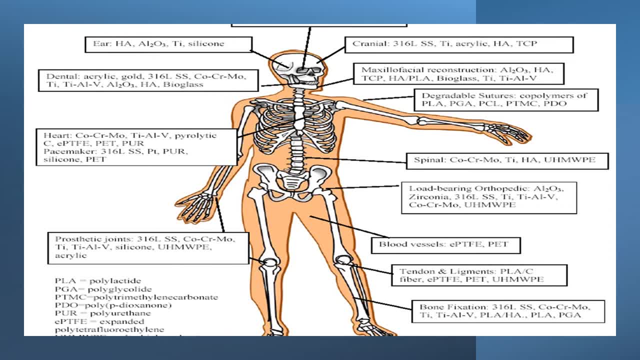 Further, for ear implants, aluminium and then titanium-silicon alloys are being used, Whereas in case of heart, which are the soft tissue, so for those titanium-aluminium-palladium alloys and then silicone-based, PET-based materials are currently being explored. 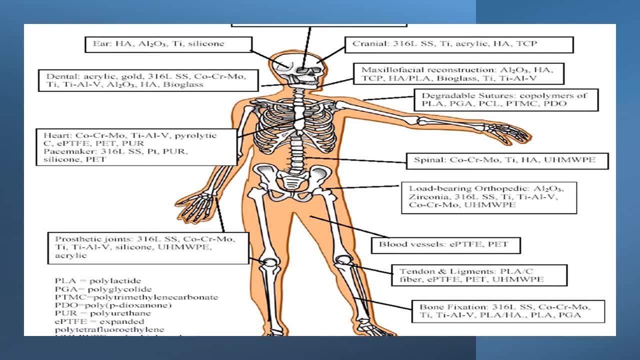 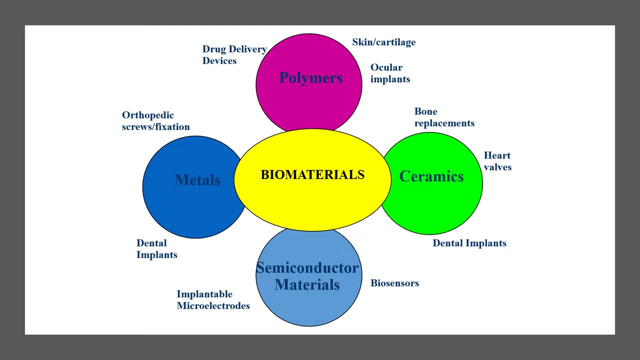 So this slide gives an overview about the various biomaterials that are currently being utilised and also gives research is being going on for further developments. so biomaterials can be of several types. majorly, it can be polymer, it can be metal, it can be ceramic and it. 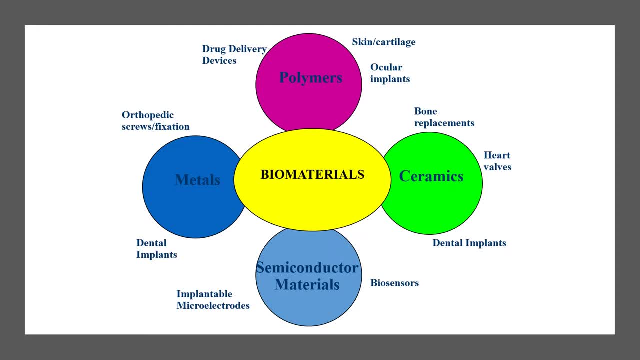 can also be semiconductor materials. so it can be utilized for various applications, namely for our devising or for developing drug delivery devices, then dental implants, then biosensor for, then also for bone replacement, heart valve, oculate implants, orthopedic screws and fixation dental implants. so 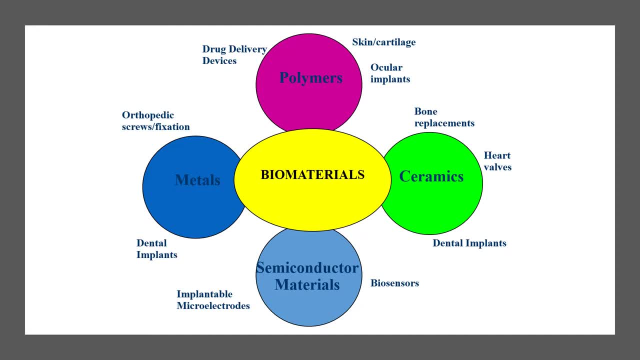 there can be several and infinite number of applications into which the biomaterials can be tuned and can be utilized for medical purposes. talking about several generations of biomaterials, so generally there were three generations of biomaterials. so generally there were three generations of biomaterials. so generally there were three. 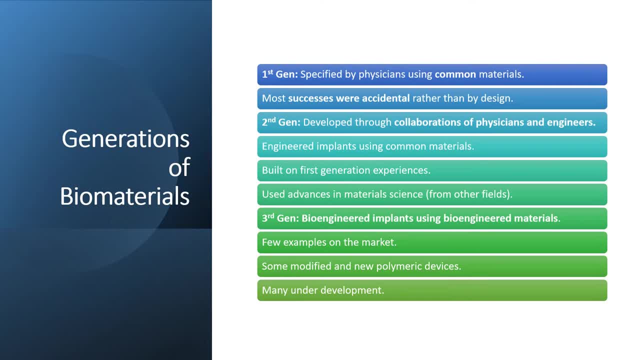 main generations. the first generation includes this one specified by the physicians by using common materials, and they were the most successful ones and they were like accidental rather than by design and by research. then comes the generation or the evolving of the second generation, biomaterials, which were 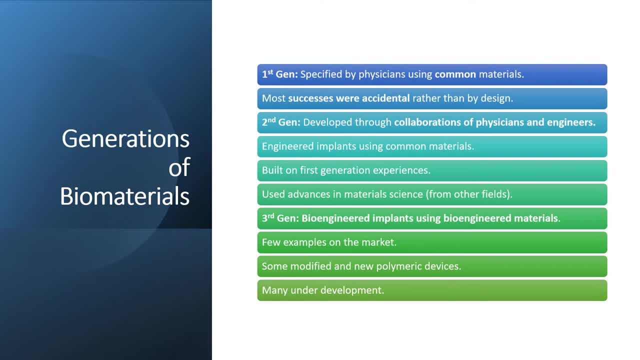 basically developed through collaborations of physicians and the engineers, and then the second generation biomaterials, which were basically developed through collaborations of physicians and the engineers, and the engineered implants were used by using common materials. so they were basically built on our first generation experiences and they utilized advances. 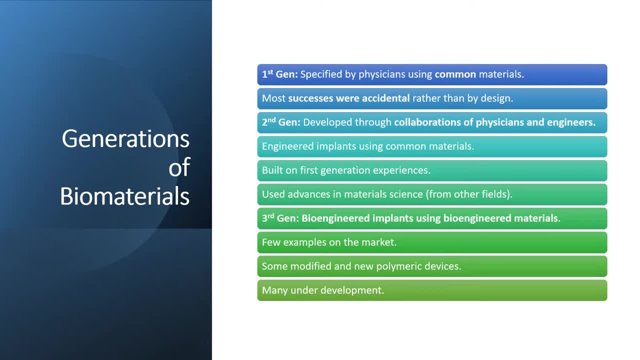 in materials science, that is, from other fields. further, the last generation of the current generation is the third generation, biomaterials, which are basically the bioengineered implants by using the bioengineered materials for a few examples on the market. so there are certain modified and new polymeric. 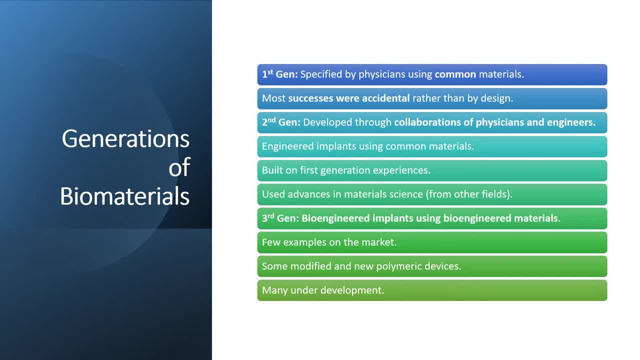 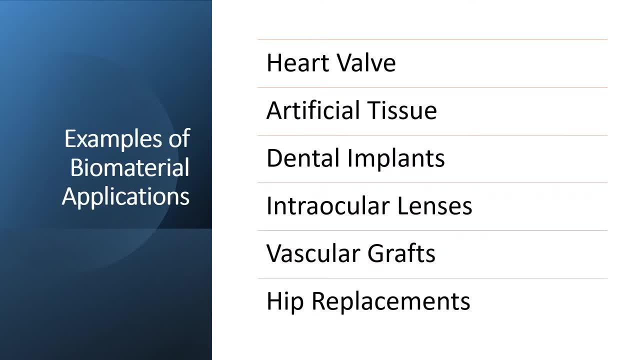 devices and they are, like others, are mainly under the development of process. talking about certain examples of biomaterial applications. so it can be utilized to fabricate an artificial or an in vitro hard valve, then it is. it can be also created, used to create artificial tissues, dental implants in. 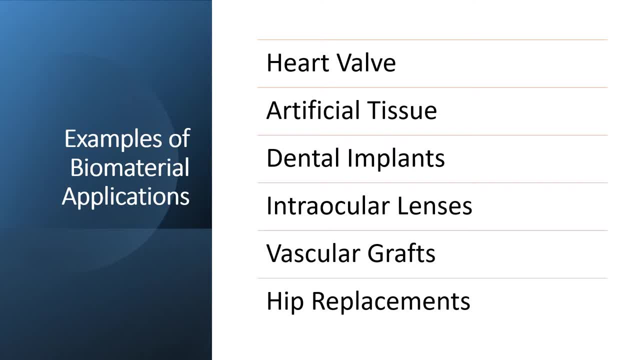 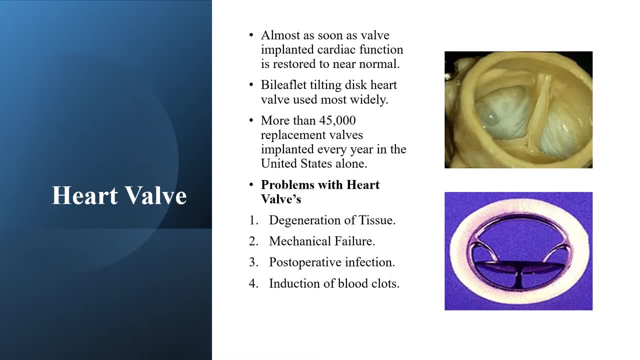 general and in臨時的 ambgesi centers for rare bone prosthetic research, for intrac Ochular Lenses, vascular grafts and also for hip replacements. going into little bit details about the heart valve, so almost as soon as a hard valve is implanted, so cardinal function is expected to restore to near a normal range. and by 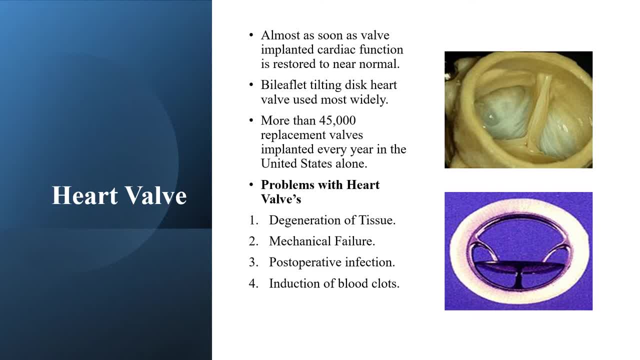 earlier Tittling Disc Heart Valve is most widely used to supply mouth besides their captores, And it has been seen that there were around more than 45,000 replacement valves that are being implanted every year in the United States alone. Further, apart from the advantages, there are certain problems that arise due to using the hard valves, which include that there is degeneration of the tissue. 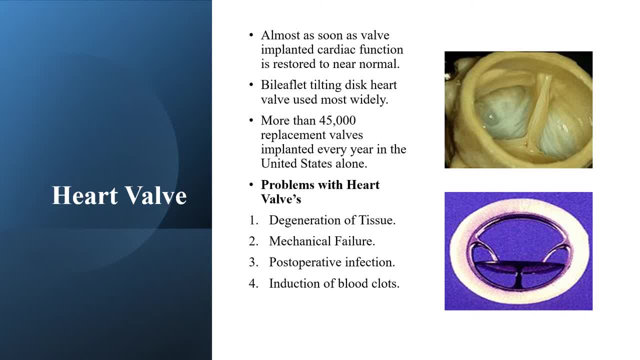 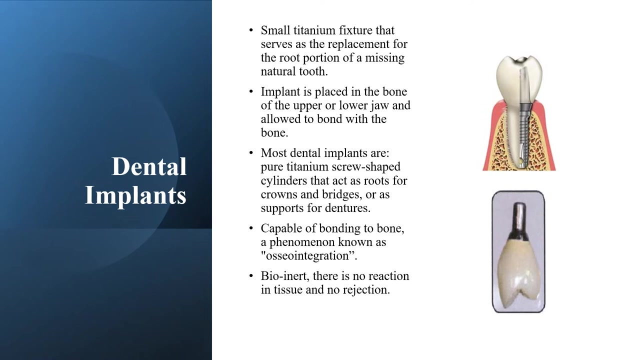 Then mechanically it is not competent or it does not mimic it mechanically. So there are several mechanical failures. Also there are high chances of post-operative infection And also there are chances of induction of blood clots. Further talking about the dental implants, after the cardiac implants, 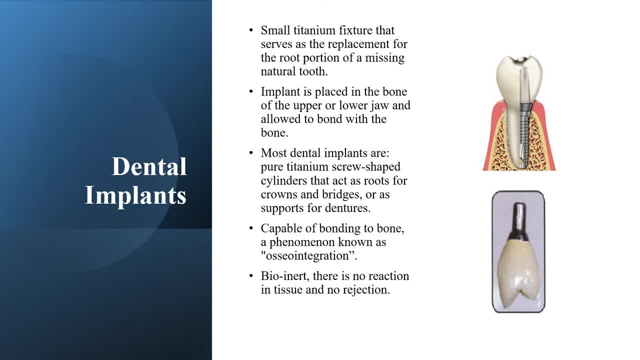 So small titanium fixtures That serve as a replacement for the root portion of a missing natural tooth. So basically, the implant is placed in the bone of the upper or the lower jaw And they are allowed to bond with the bone. Further, several dental implants are basically based, or like made up of titanium screw shaped cylinders. 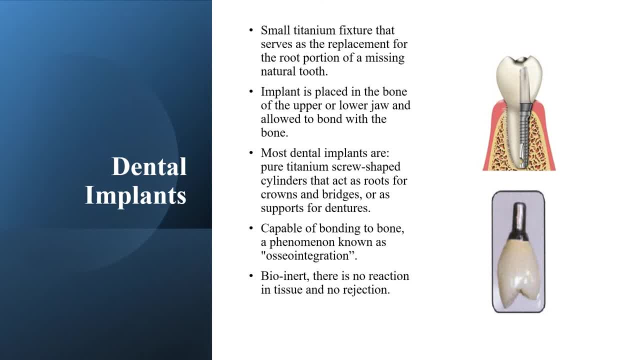 That can act as roots for the crowns and bridges, Or also can act as supports for dentures. Further, they are also capable of bonding to the bone, Which is a phenomenon that is termed, or that is described, as osseointegration. 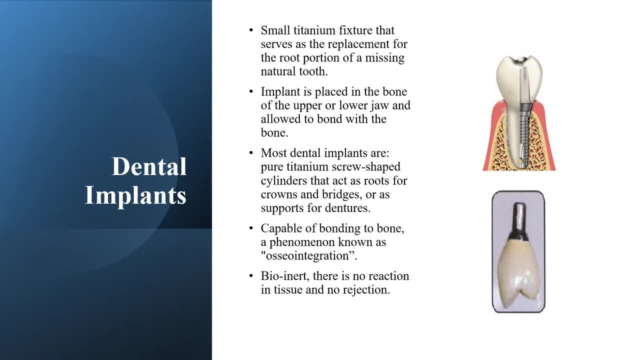 So for any material that are being used for dental implants should have been featured of the osseointegration And they are also bioinert. Thus there is no reaction in the tissue. And also there is no reaction in the tissue. 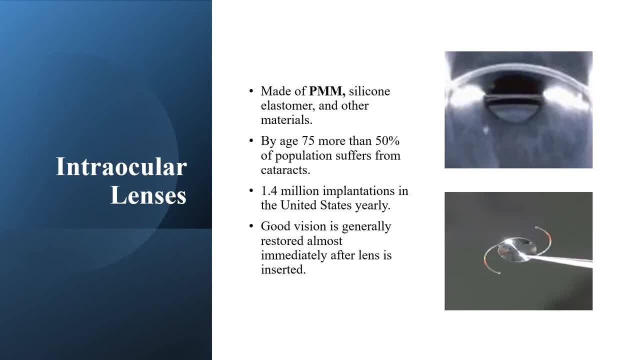 And also there is no reaction in the tissue And also there is no rejection of it. Talking about intraocular lenses which are currently ​​being really explored, So basically they are made up of PMM and other such materials. So by the age of 75, it has been observed that more than 50% of the population 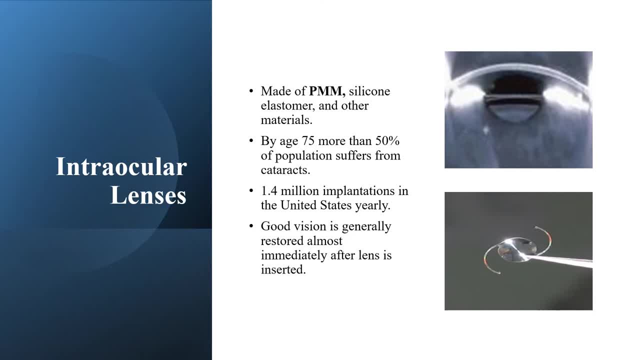 they tend to suffer from cataracts. So people are, like, mostly seen having problem in the vision. So people are, like, mostly seen having problem in the vision due to the cataract, and around 1.4 million implantations in the united states are being 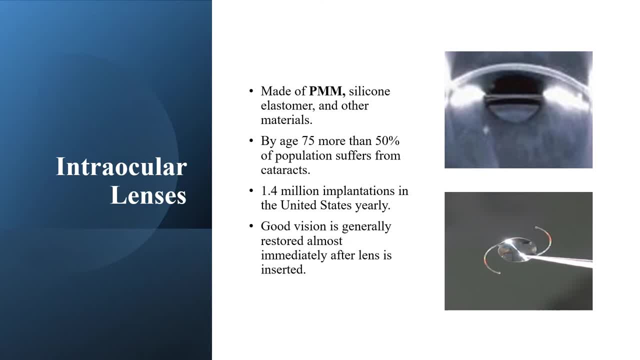 done like on a yearly basis, and good vision is tend to generally get restored almost immediately the surgery is being done or after the lens is inserted. so this shows that how tissue engineering and regenerative medicine has evolved and how they are being utilized to improve the quality of several patients all throughout the world. thereafter talking, 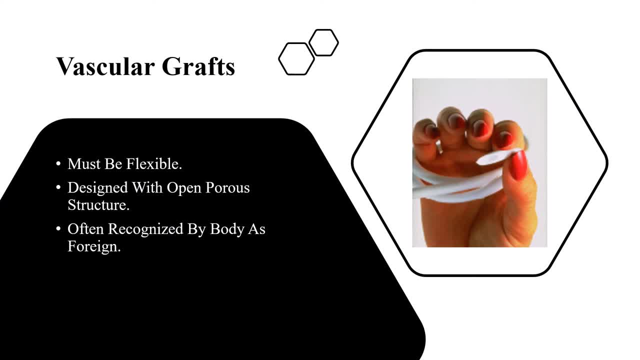 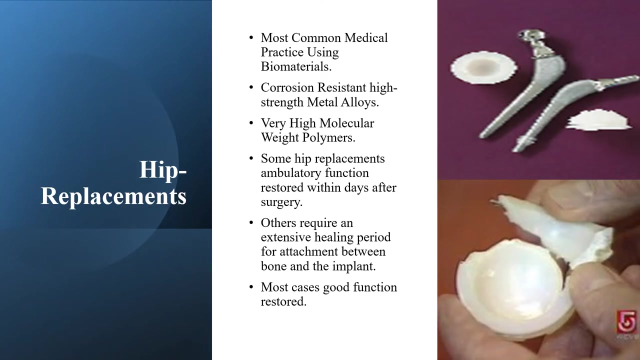 about vascular grafts. so vascular grafts as a name would suggest that they need to be flexible in order to be utilized as vascular grafts, and they are generally designed with the open porous structure or nature and they are often recognized by body as a foreign. next, discussing about what hip replacements are and a certain brief overview about it. 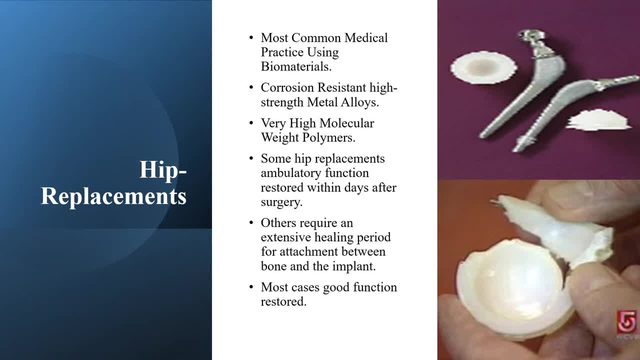 so in biomaterials. the most common medical practices using biomaterials in this case is like: it should be corrosion resistant, it should have high strength, it should be made up of high strength metal alloys. so a very high molecular weight of polymers are being utilized, because it is an area which 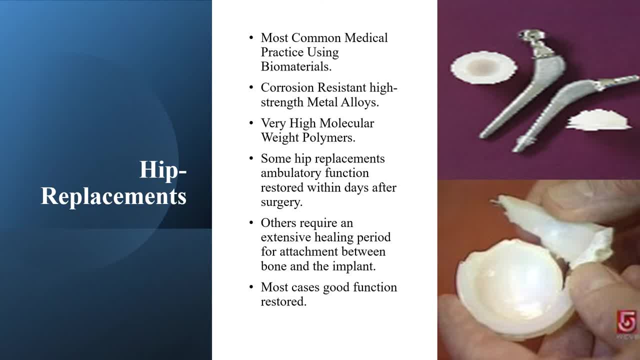 experiences higher body weight and other pressures and all those- so basically some hip replacements are ambulatory function- are tends to get restored within certain a few days after the surgery and other surgeries. they basically require an extensive healing period for attachment between the bone and the implant. so in most of the cases 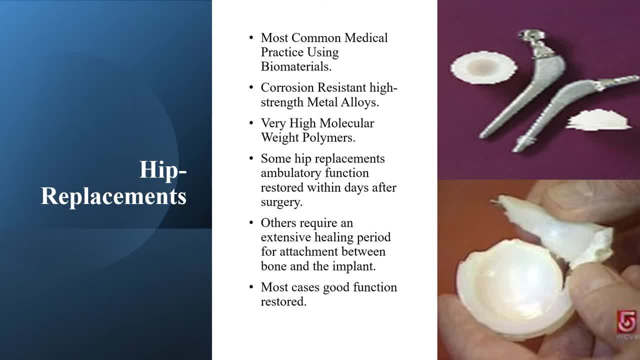 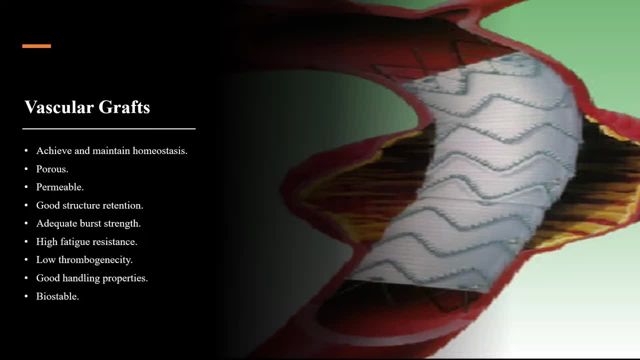 good function is being restored at a rapid manner. so, talking about vascular grafts, and what are the characteristic and characteristic features that are being required for vascular grafts are? so? basically, they should be porous, they should be permanent spines, they should be flexible and they are not necessary to. 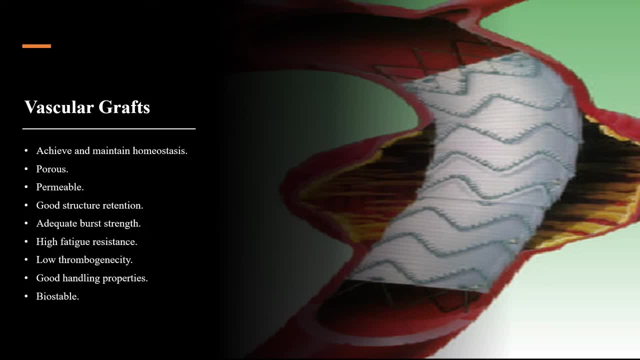 permeable. they should achieve and maintain the homeostatic balance that is normally maintained in our body. so it is a one of the most important points to be kept in mind while designing or fabricating vascular grafts, as it should maintain the homeostatic and balance and nothing extra or 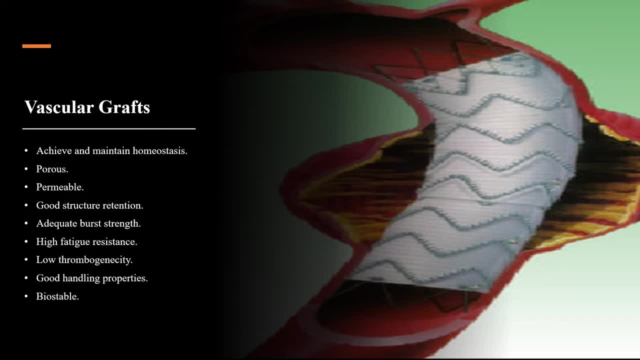 nothing a hindrance to the process of maintaining the homeostasis should be disturbed. so it should also have certain of good structure retention abilities and adequate burst strength, along with high fatigue resistance, low thrombogenicity, and it should be biostable, apart from other good handling of properties. so these are a few of the 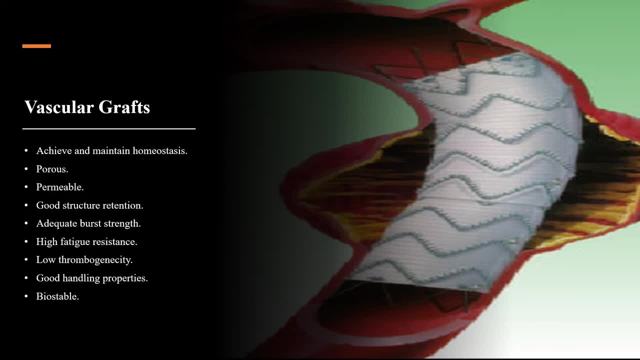 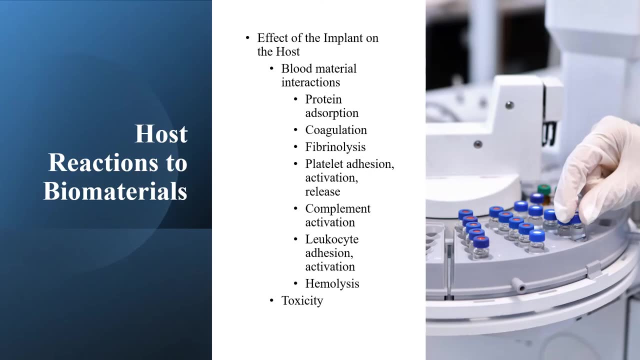 parameters that are required to be kept in mind while designing vascular grafts. so, although these biomaterials are like, they don't elicit that much immune response, but still there are certain responses between the host and between the host and the implant. so the first reaction, 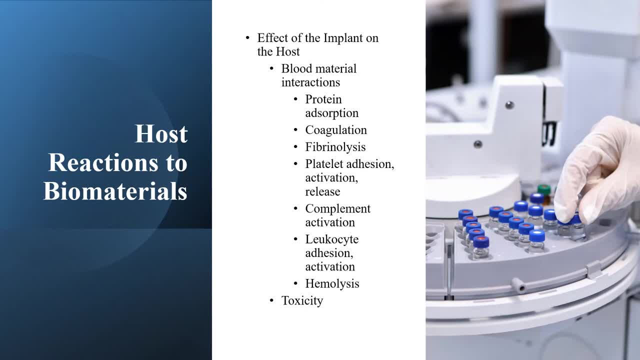 that happens is the blood and the material interactions, basically due to the protein adsorption, then coagulation, fibrinolysis and the other factors that are involved in the process. so then hemolysis, then there are certain adhesion and activation of nucleosides, then there's 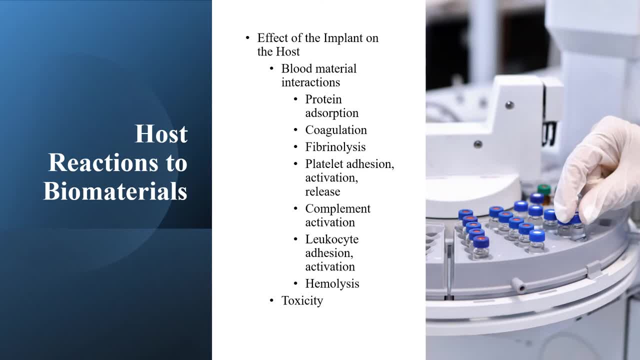 also activation of the complement system of the immunological pathways so that results into the adhesion of the platelets, also activation and its release. so basically when any biomaterial or any scaffold is implanted into the body. so the first, there are several of thousands of protein. 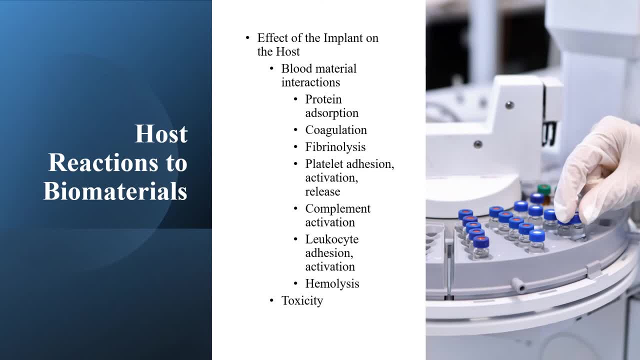 absorption. so it can. it can be used to easily create a complete clonal structure and it can. that takes place before we do anything else. so there are certain parameters, so basically the cells. they are not that in direct contact with the material, but with the cells that 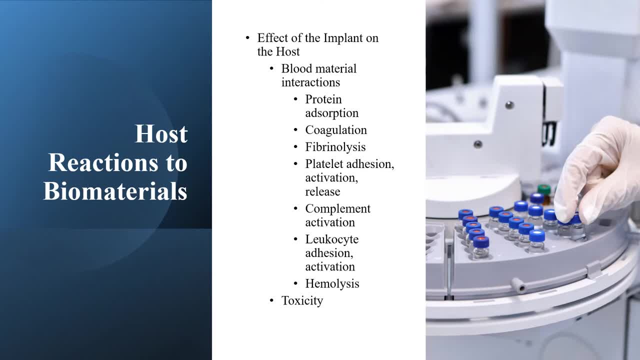 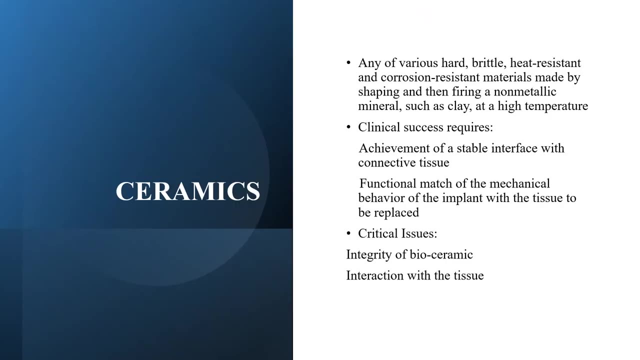 covered the material. so basically these are few of the major reactions. apart from these, there is also chances of toxicity, so that can also be assessed from this. further talking about what ceramics are and why it is being used and what is the main area for it to be utilized, so any of the various hard then brittle, heat resistant and corrosion. 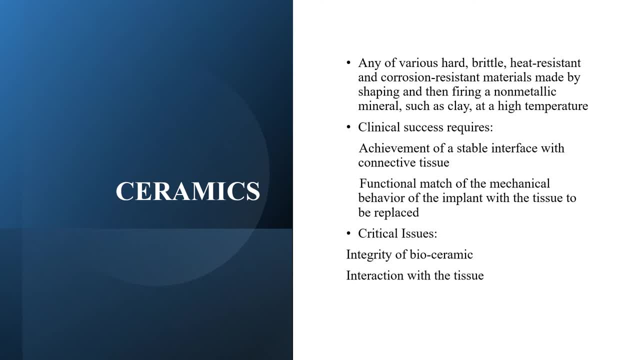 resistant materials that can be made by a shaping and also by firing a non-metallic mineral such as that can be a clay at high temperature. so The main point is that it requires a clinical success and clinical success in turn returns required, certain achievement of a stable interface with that to the connective tissue and also 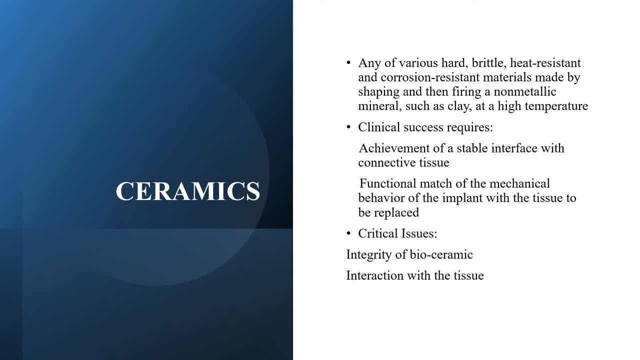 it should have the functional match of the mechanical behaviors. the mechanical attributes should be able to be like mimicked and also when implanted'll get the functionally本 aus, also when implanted, like mimicked and also when implanted, the functional match in that mechanical behavior. 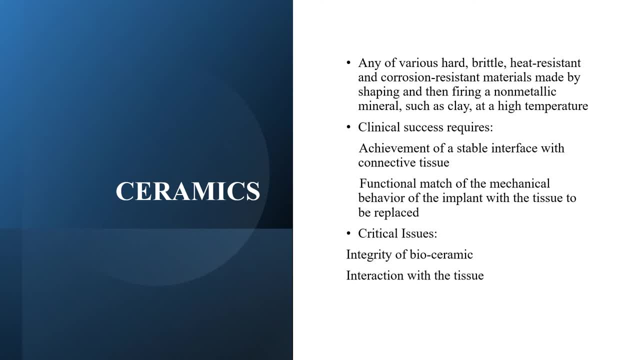 So it requires a structured structure which have the structure of a person and also it should behave like, in that it is in the in vivo or the native condition, and also behavior of the implant with the tissue that needs to be replaced is needs to be studied. then there are certain critical issues like integrity. 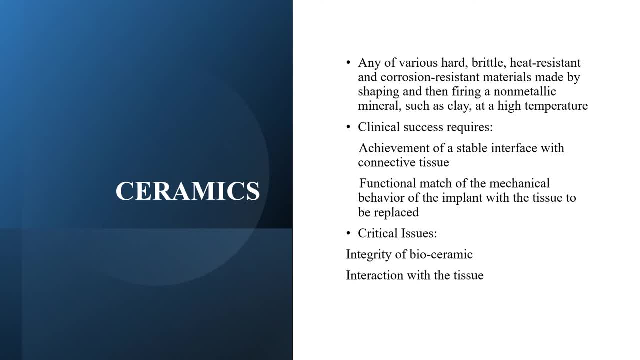 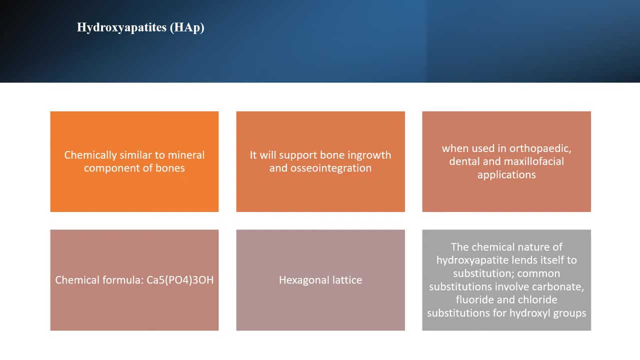 of the bioceramic and also interaction within the tissue. so when talking about ceramics, the first and the widely used material that comes into mind is hydroxyapatite. so it has several advantages to be used as a semen for bone tissue engineering purposes. some of its major and worthy 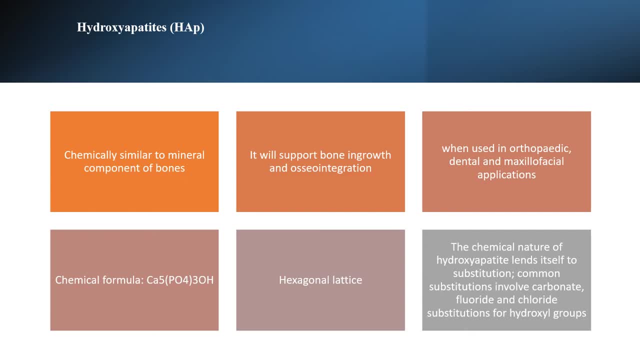 advantages include that they are chemically similar to mineral component of bones and they also support of the in growth of bone and also allows of for the osseointegration. as I've already mentioned what osseointegration is. as I've already mentioned what osseointegration is, 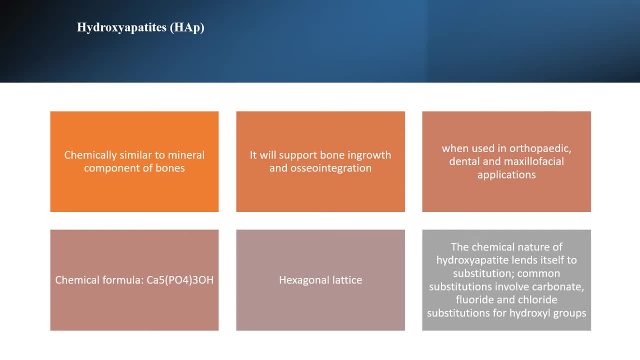 in my previous few slides and also um. they are used in orthopedic or dental and maxillofacial applications and they are clinically being utilized and explored. and even all over the world research is being going on to develop further specialized and doped and functionalized of. 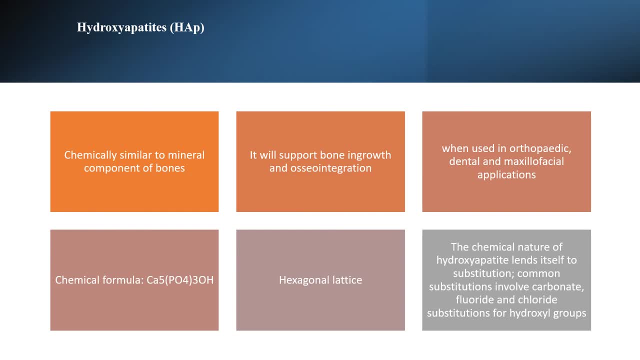 hydroxyapatite for specific uh like, for specific function observance. so basically the um chemical formula is being shown onto the screens and apart from these uh, so basically these have the hexagonal lattice structures and uh, the chemical nature of the hydroxyapatite. they basically they tend um itself to a substitute or the common substitutes. 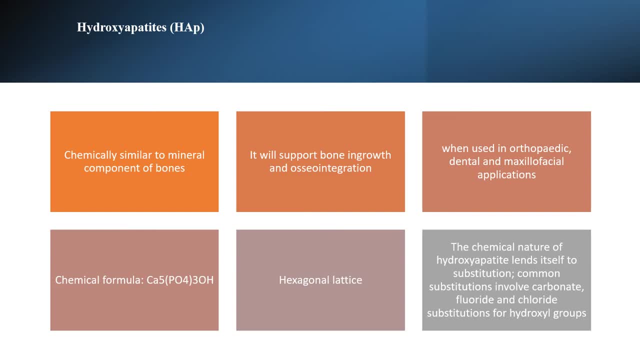 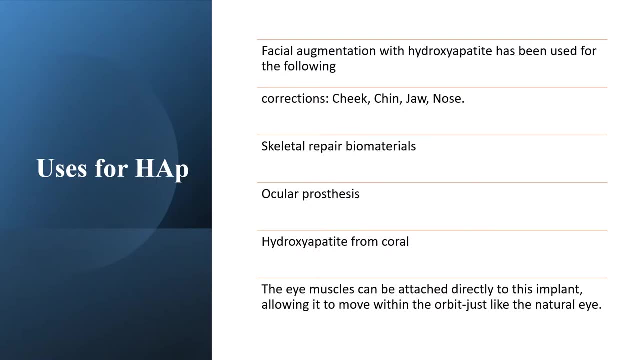 involve the carbonate, the chloride and a chloride substitution that is required for the hydroxyl group. so there can be several applications and utilities or uses of hydroxyapatite, which is also known as hap, so it can be utilized for the facial augmentation with hydroxyapatite that. 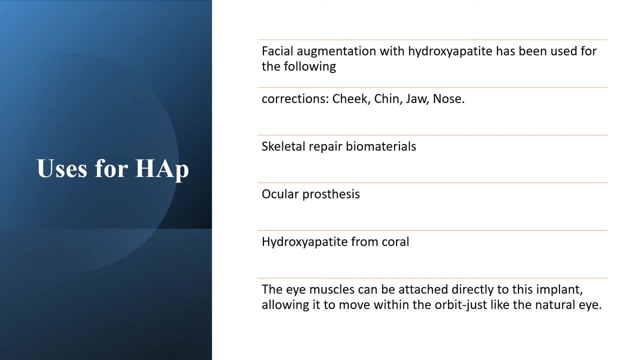 has been um used for the following corrections: uh, like it has been used for the cheek correction. um, then cheek correction, jaw and then also nose correction jobs and also a skeletal repair. biomaterials, then other materials like the ocular prosthesis and hydroxyapatite from coral. 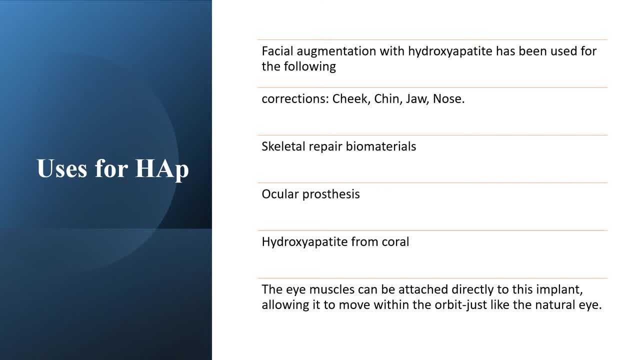 so, basically, the eye muscles, um, can be attached directly to the implant, allowing it to move within the orbit just like the natural eye. so, uh, this gives an overview about the versatility of the hydroxyapatite and how it can be modified in order to tune it according to the desirable function that needs to be observed. 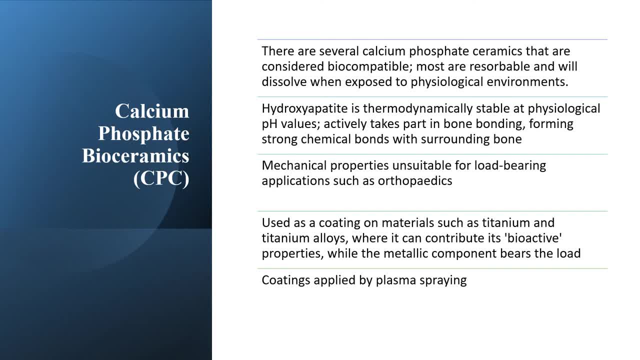 apart from using hydroxyapatite, another widely used material in this field is calcium phosphate bio ceramics, which is also written as cpc. so basically, there are several calcium phosphate ceramics that are being considered biocompatible, and most of our of them are bioresorbable. 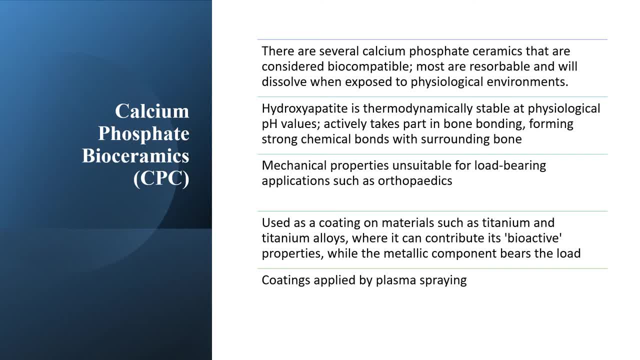 and will, uh like, tend to get a dissolve when exposed to physiological environments. so that is one of the desirable characteristics, uh, that jishu engineering has and how it really encompasses that portion. so, uh, basically, um, talking about it, so hydroxyapatite is a thermodynamically stable polymer at physiological ph values, and it also 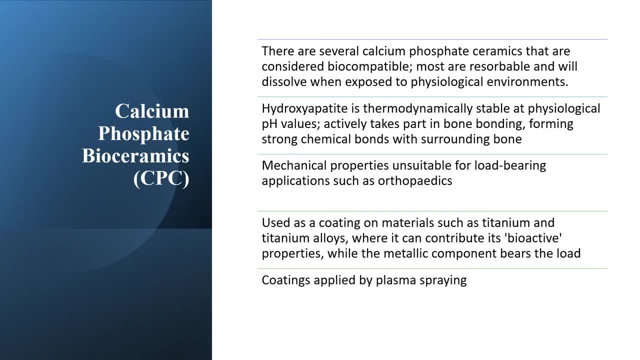 actually takes us part in the bone modeling um, then also the forming the uh strong chemical bonds, then it also leads toward the mechanical properties that are really unsuitable for the load bearing applications, which includes the orthopedic application, and also it can be used as a coating on materials such as titanium and titanium alloys, so basically where it can. 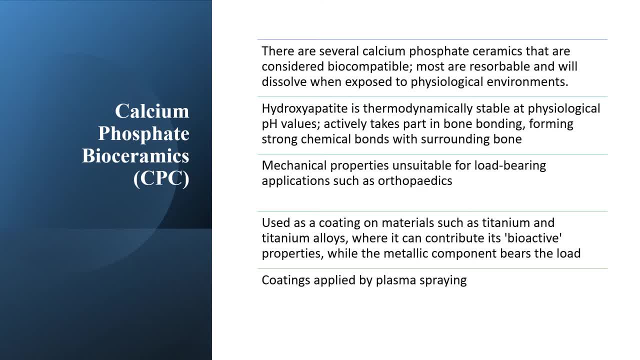 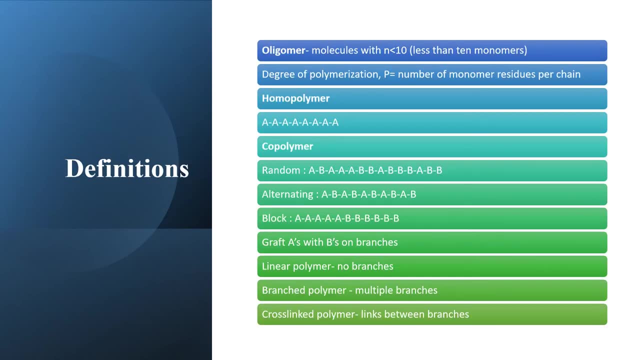 contribute its bioactive properties, while the metallic component appears, the load. so there are certain coatings, like by the plasma spraying, that are also being utilized and also being explored by researchers. further, talking about several definitions and how the biomaterials are synthesized, so they are basically the oligomers. so oligomers are the molecules. 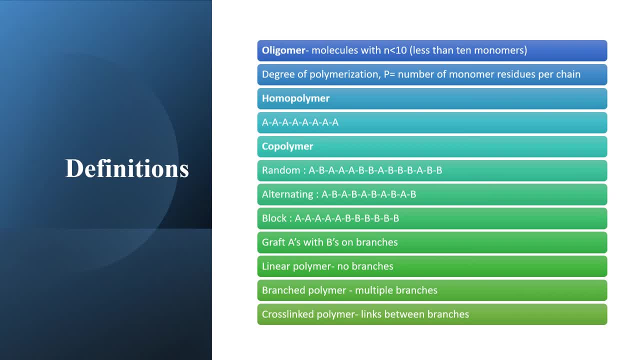 with N or the number of which is like the number it should be, not like it should be, be around less than 10, but not more than 10, and there are also certain parameters like the degree of polymerization. then, apart from those, there can be different types of biomaterial depending upon. 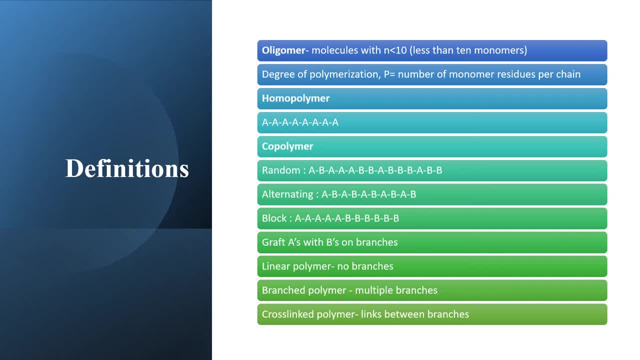 the synthesis process, so it can be either a homopolymer or a copolymer or it could be alternating, block, random polymer and also linear polymer directly can be utilized which doesn't have any of branches and also there are certain cases where there are. they use. 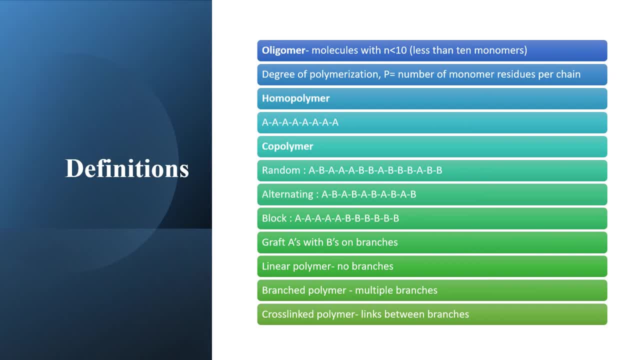 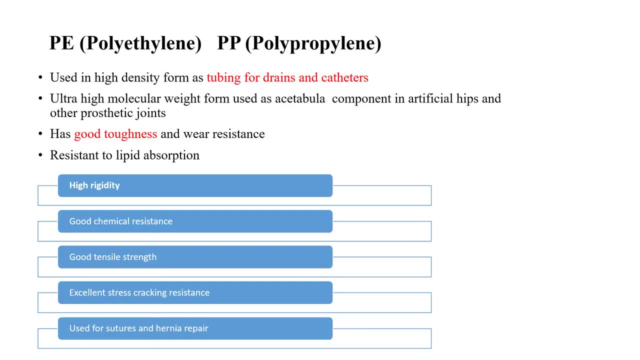 the branched polymers for it. so these are certain um definitions which i'm going to discuss. one of the major examples include the polyethylene and the polypropylene. so basically, they are used in the high density form and they are used to fabricate the tubing for trains. 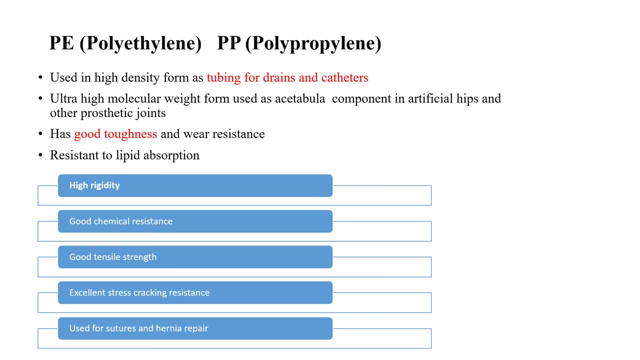 andๆ. no injectors are needed if a fuel is supplied for the designed work and solutions are א स dynasty form and they are used to fabricate the tubings for trains and also for the catheter of application. so basically, these are the ultra high 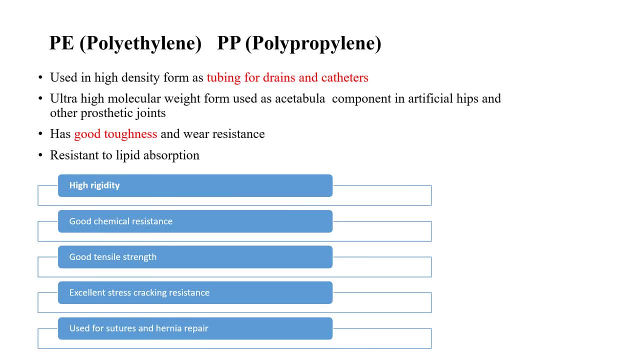 molecular weight, a form that are used as acetabular component in artificial hips and also for other prosthetic joints. so basically it has good toughness and water resistance. so different materials has different properties, so a people need to choose the desirable material depending upon their use and depending 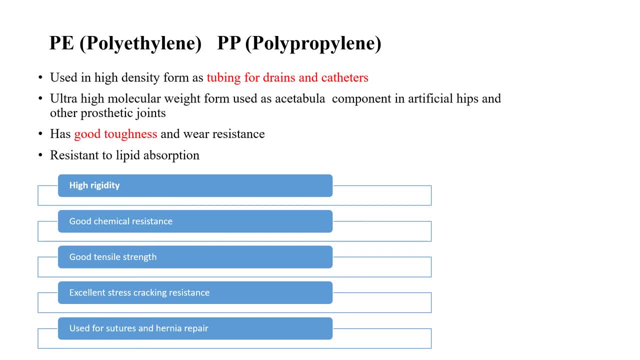 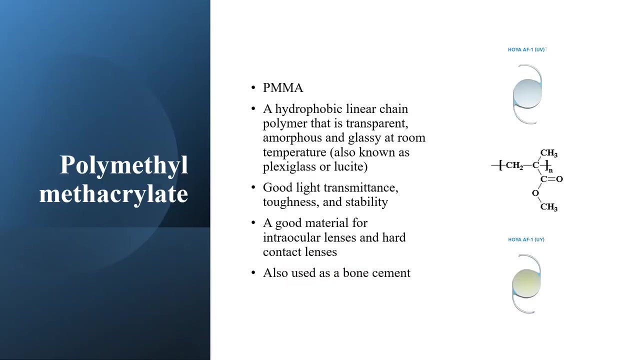 upon their application. so basically they have high rigidity. then there is a good chemical resistance, and also they have, they possess certain good cutaneous strain and then also there are excellent stress of cracking resistance stuff which are used for sutures and also for ania, are prepared further. next we discuss about the polymethyl. methyl勝 react, which is dude, as i have mentioned잡lich, where it is obtained by清 ce la wh and diluted by tarsalzeane. sticking out of Givenchy and hypolysis, doctrine of today is which lies on the inca had to be. 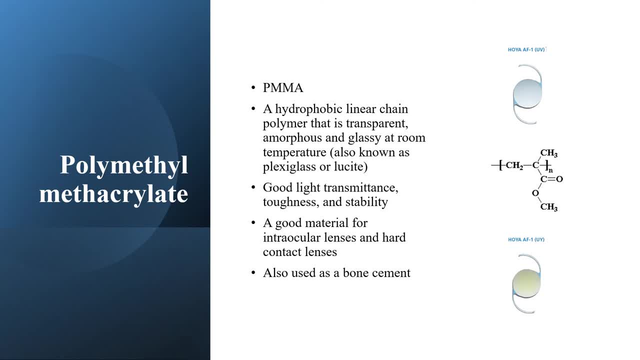 third, wonders of its application. aboutingly, after the application of osteo dent, Creates the formula which is most important, structure, and how this happens is also known as PMMA, and so basically talking about its definition and a brief idea. so these is actually hydrophobic linear chain polymer, that is, tend, that tends to be transparent, amorphous. 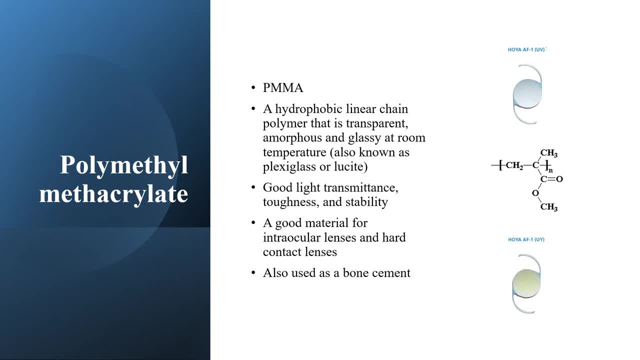 glassy at room temperature and they're also known as a plexiglass or lucite. further, there can be good light transmittance, then toughness and stability, and they are also considered as a very good material for the application of hard contact lenses and also for intraocular lenses. 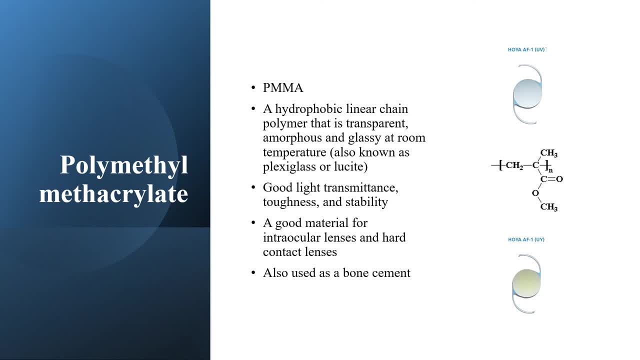 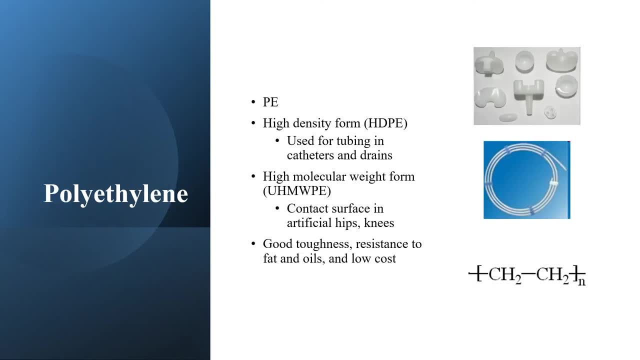 apart from these, they are also utilized in the foundation engineering and they are basically used as a bone cement. next, talking about the polyethylene, so they are basically dyes in a high-density form, or which is known as HDPE, and they can be used for fabricating tubings in catheters and also in the drains. so certain high molecular 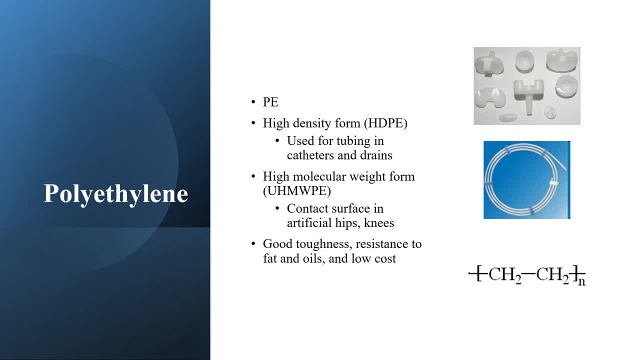 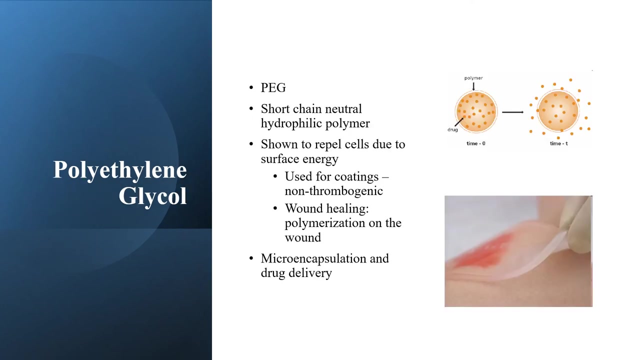 weight form. they actually, for example, the contact surface in the artificial hips and knees and they basically they have good toughness. then our resistance is there, resistance to fat and oils, and they are also of a minimal cost. so these are certain advantages of using it. further, talking about the polyethylene glycol, so these are also known as PEG. so basically, 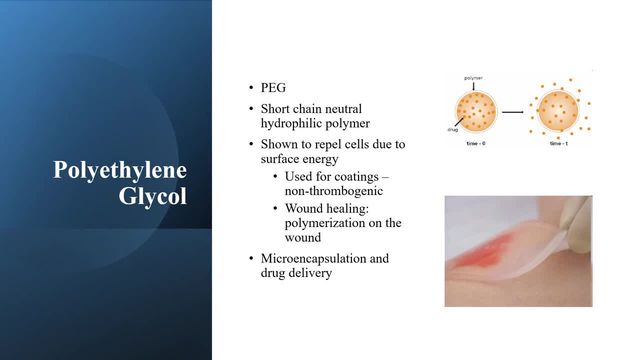 these are the short chain polymer, hydrophobic polymer based materials and they are basically shown to come to pale cells and typically these are no, so those are a very common one and we can due to surface energy, and they can be used for either coatings or non-thrombogenicity. 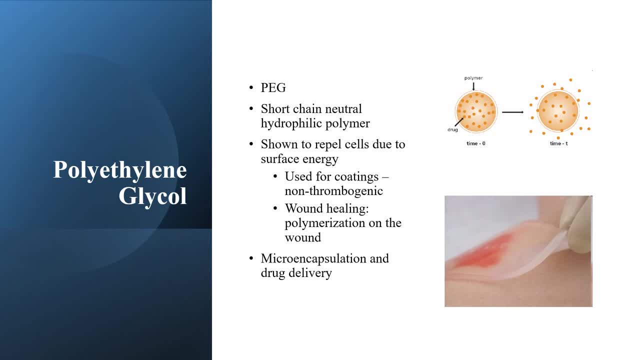 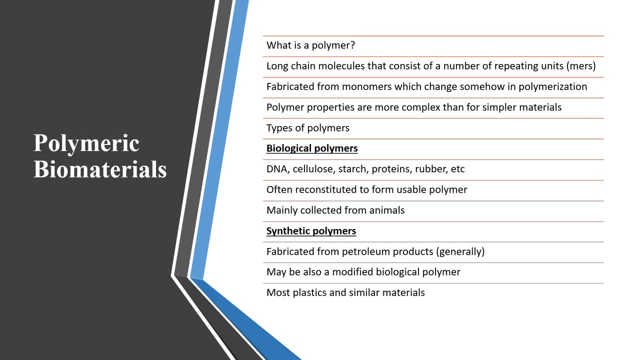 and also they can be utilized as the for the wound healing purposes and polymerization on the wound. further, they can be utilized for the micro encapsulation and also for drug delivery purposes. then our next. we'll be talking about certain biomaterials which are of polymeric origin. 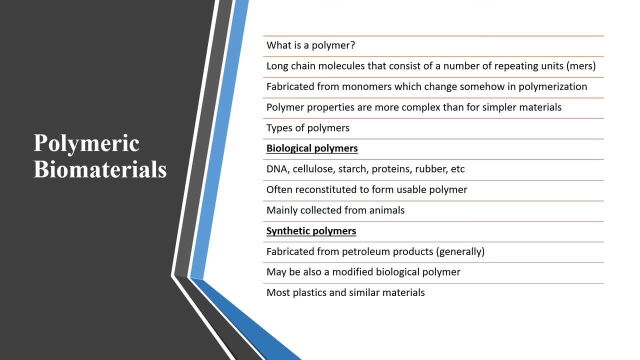 so now we can have a question in our mind that what is a polymer? we know what is a biocompatible or biomaterial. now we'll talk about what polymer is. so, basically, these are the long chain molecules that comprises of several number of repeating units based on the designing and requirement. 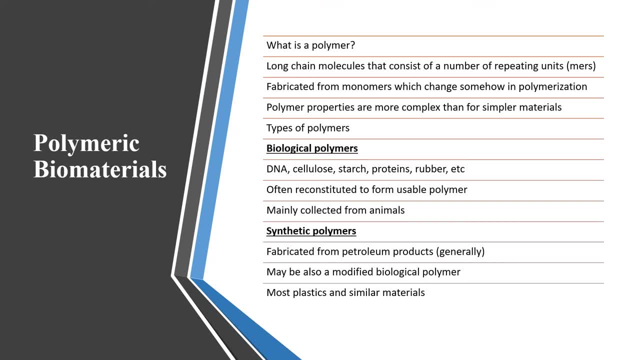 of a particular biomaterial. so we can have a question in our mind that what is a polymer? so basically they are a fabricated from monomers that are generally exchange or somehow in polymer polymerization and also of the polymer properties are much more complex compared to the 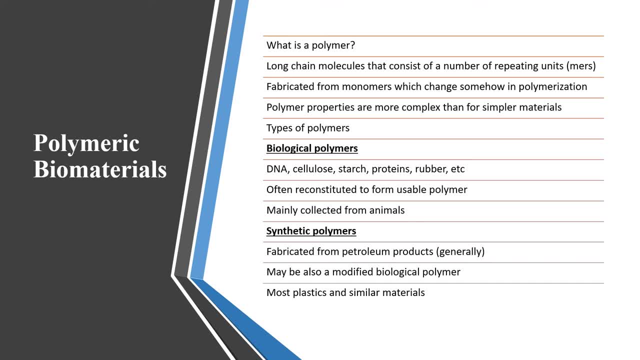 simpler materials and there can be different types of polymers. so basically the two subdivisions include the biological polymers and also are the synthetic polymers. so the biological polymers are the synthetic polymers and the synthetic polymers are the synthetic polymers. it includes the list of examples, like the cellulose, the starch, proteins- a rubber is also there. 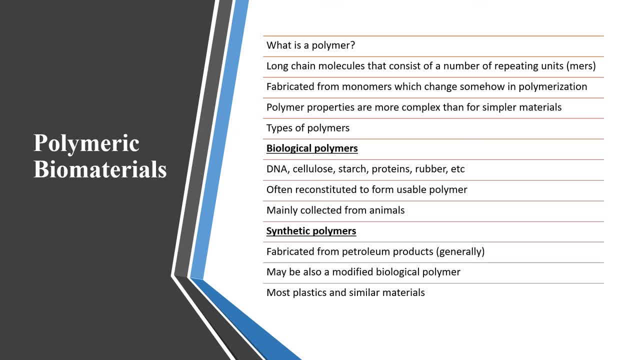 then often they are pre-constituted to form a very usable polymer, which are mainly collected from the membrane. so basically there can be synthetic polymers that are fabricated from petroleum products and generally they can also be modified biological polymer and also most plastics and the similar materials. so there are certain differences between the PTFE, which is 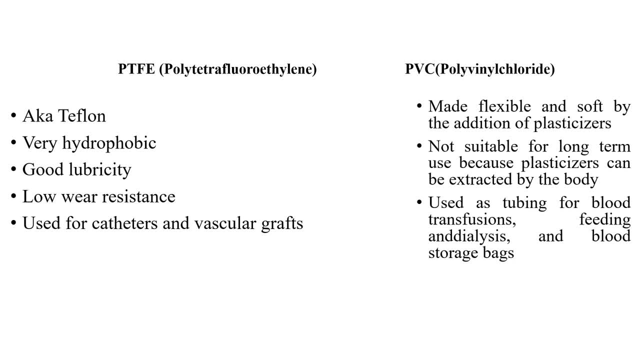 polytetrafluoroethylene and the other is polyvinyl chloride, which is also known as PVC, so they can be either the teflon or they are actually hydrophobic. they have good lubricity in case of the poly PTFE and they basically are utilized to be used. 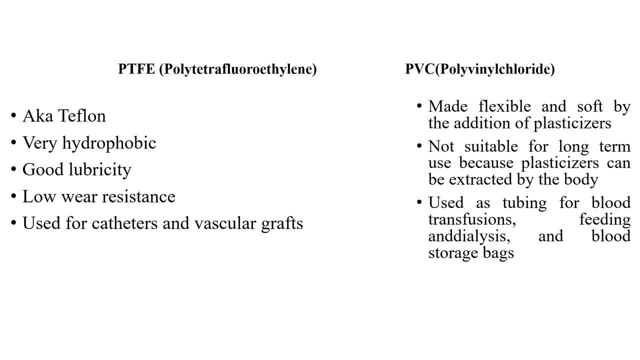 for uh fabricating catheters and vascular drugs coming to the PFC, which is polyvinyl chloride, so they are a like in general, made flexible and also soft by the addition of plasticizers, so they are not suitable for long-term use because plasticizers can be extracted from the body and 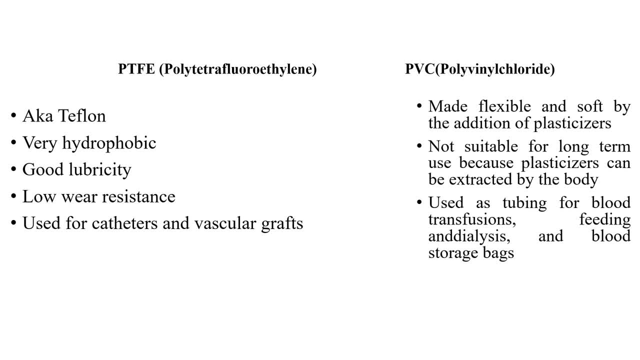 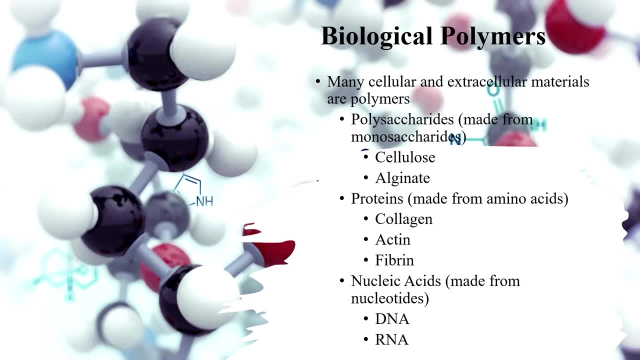 they are used as a tubing from a blood transfusions and also feeding and dialysis and also, um like, a storage bags, talking about a certain biological polymers. so basically, uh, there can be many uh and extracellular materials, um like, which are also known as the polymers, so polysaccharides, as the name suggests that they are. 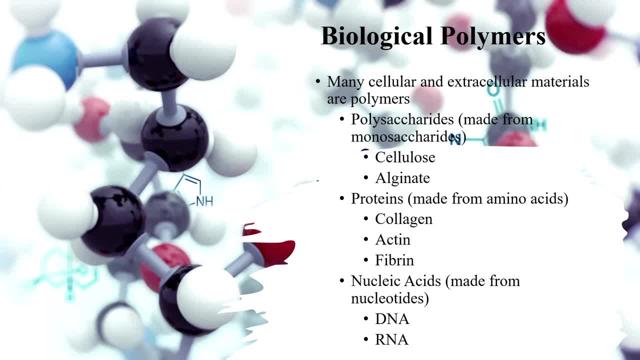 ones which are made from the monosaccharides, like the cellulose and also the alginate. so sometimes, uh, they can also be utilized as proteins, uh, mainly from the amino acids, like, for example, the collagen, then actin, and so, uh, they can be also nucleic acid. 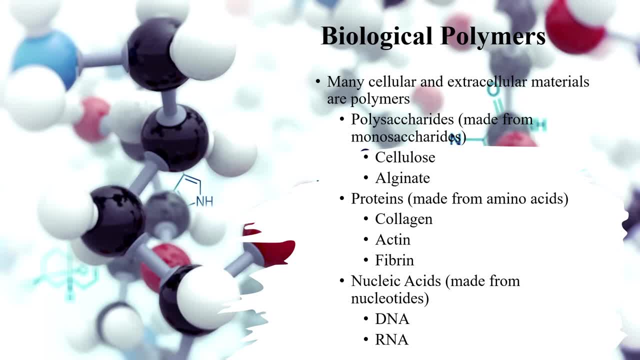 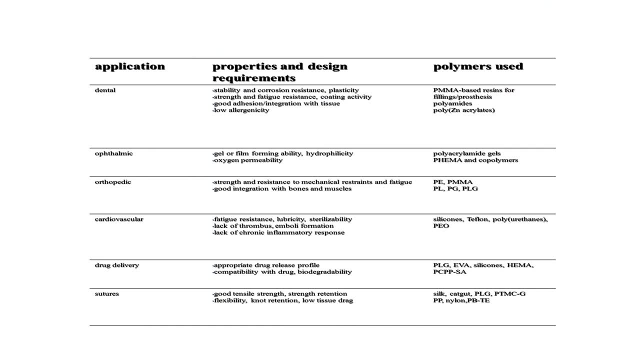 which are made from nucleonides. either that can be of DNA or it can be already further. it shows that there are several areas or domains of tissue, so it can be either gentle, then opthalmic, then orthopedic, is there cardiovascular, and then also for the drug delivery and also suture or research purposes. so this uh table or chart shows the